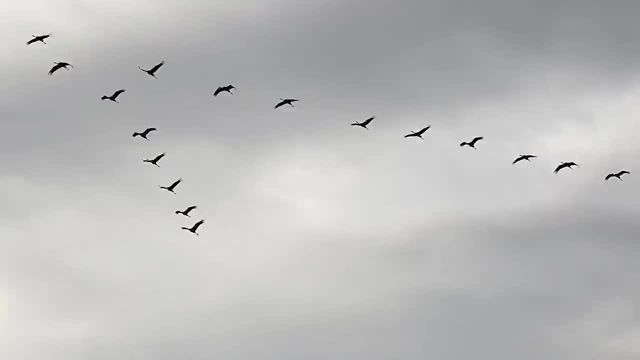 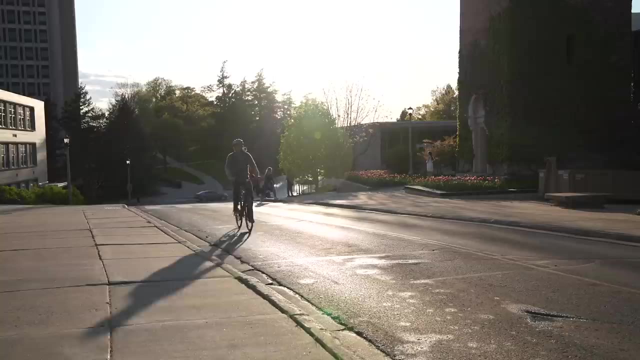 I don't really have that good of a natural spatial geometric sense. I think you're supposed to if you're a mathematician. It's like sort of those are things that are supposed to be associated, but just looking up, or sort of outside the building where I work, my office, 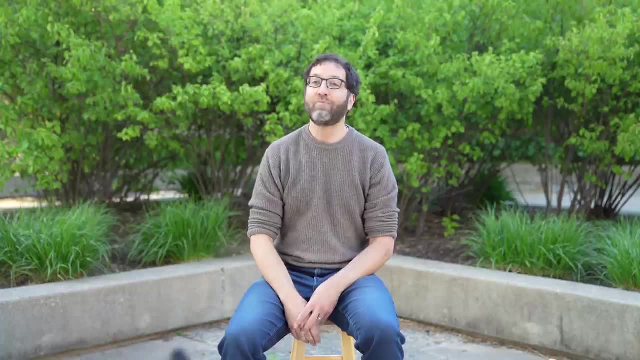 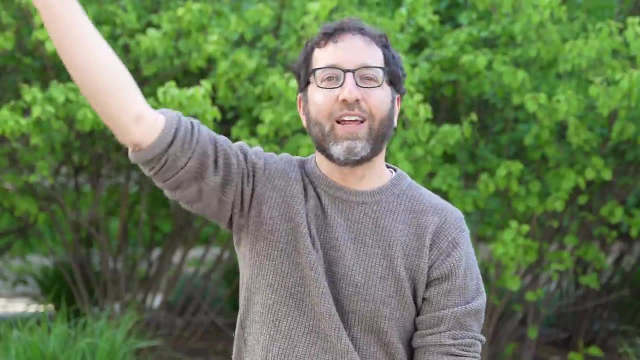 is in there somewhere, But where it is I could not tell you. I go in there every day for 15 years, but like whether it's on this side of the building or the other side of the building, or like whether it would be down there or over there, I truly have no idea. 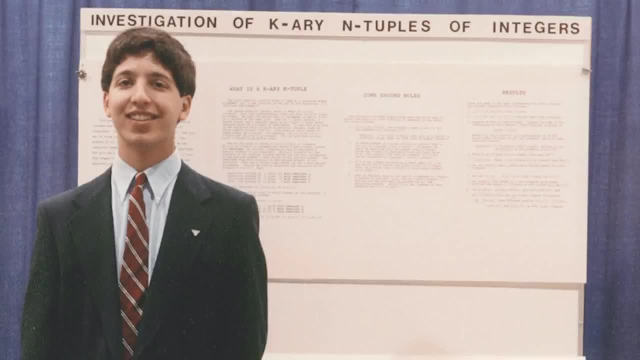 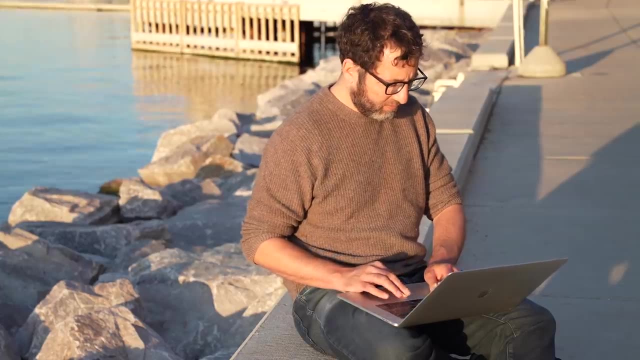 When I first learned geometry I didn't care for it. It didn't suit me And I think maybe that was part of it. I think it was only once I started to understand that algebra and numbers and geometry under the skin were the same, that they could be combined and sort of work. 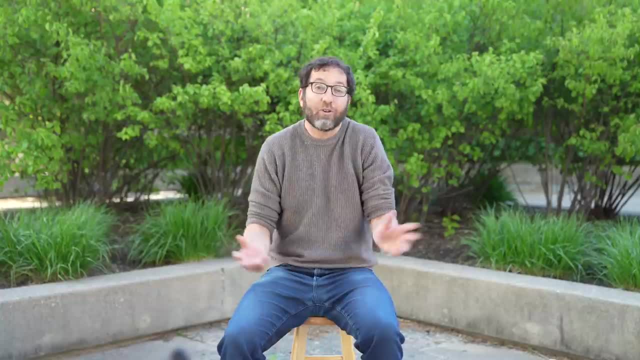 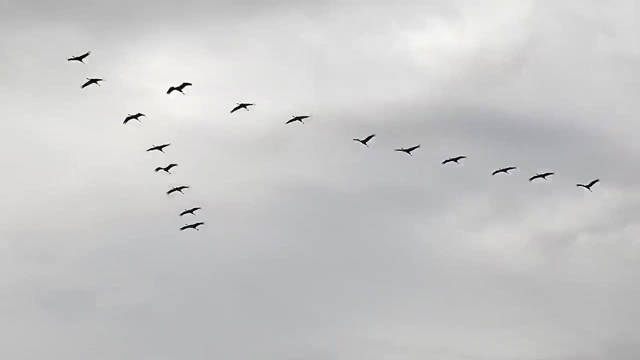 together. That was my way in. I still don't know where my office is. If I'm inside, I can find it. don't worry, I know the number. That's how I find it. Geometry is everywhere. Any kind of game. 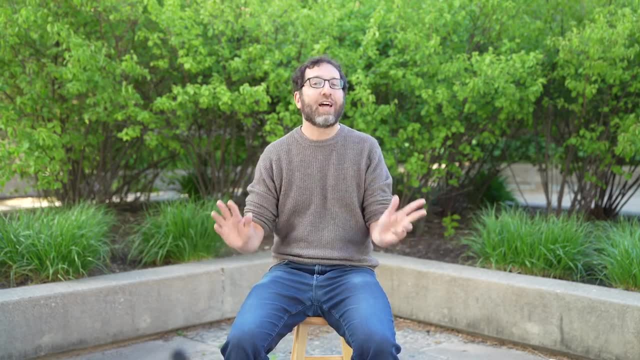 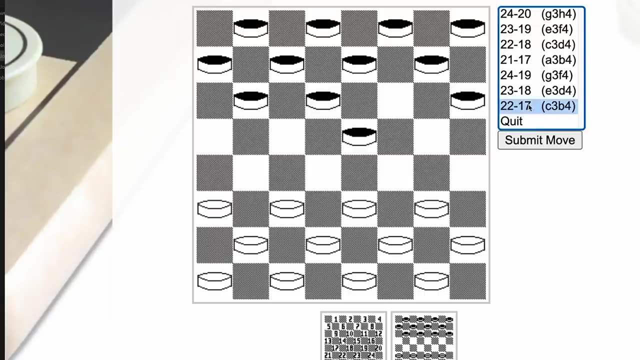 whether it's checkers or tic-tac-toe or connect four or chess or go or whatever, the game itself has a geometry And when you train a machine to play that game, you're training the machine to explore that geometry, And that geometry is the geometry of a tree A. 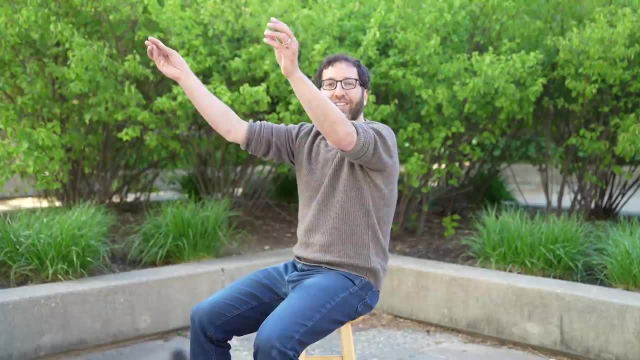 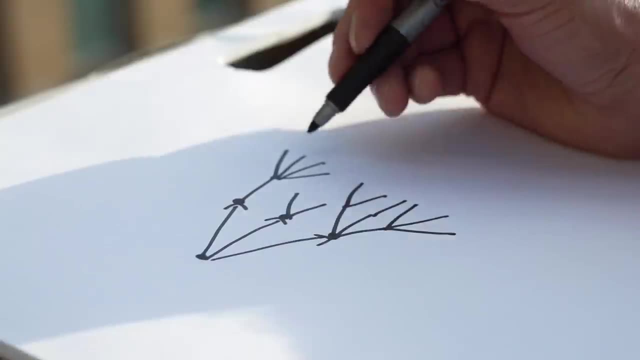 tree, depending on which one you look at, it has a trunk, and that trunk branches into smaller branches and the small branches branch into smaller branches, and et cetera, et cetera, et cetera. But you can never go back right. That's the way a game works. That's the way 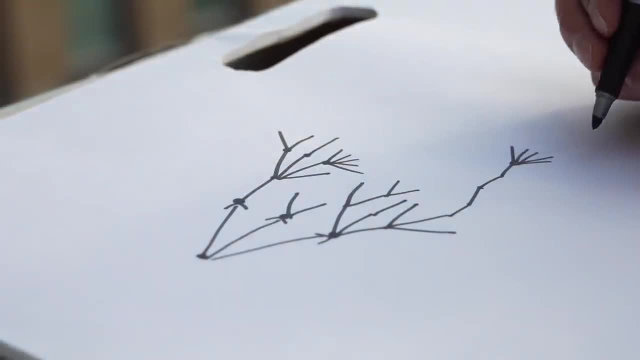 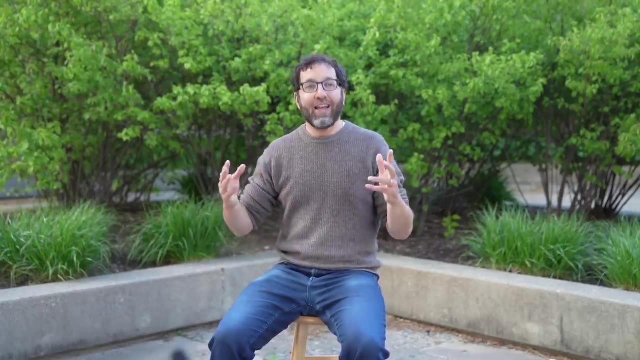 any kind of linearly sequenced set of decisions works. It's the tree-ness of the geometry that makes those games solvable. That's what makes it possible for there to be a literally perfect strategy, which is what we now have in computer. 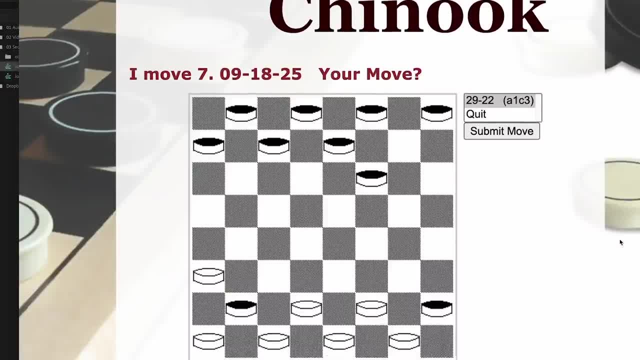 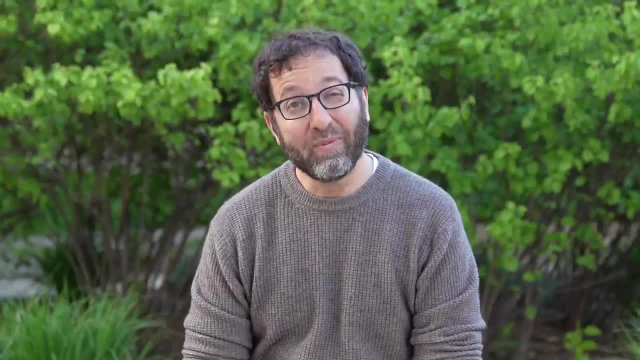 checkers So you can play. you know you can play against the computer. It's just sitting there at the University of Alberta running all day and night and you can log in and play against it At some point. usually it takes about three or four moves for me, because I 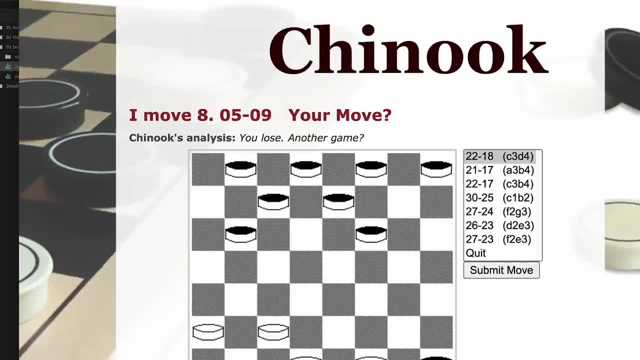 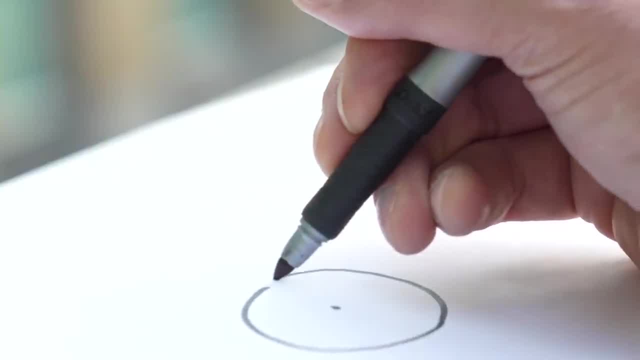 don't really know checkers very well, It'll just be like I have one. If what you know about geometry is like three or four moves, it's like I have one. If what you know about geometry is like ninth grade, it doesn't seem like it could be very dangerous, But there's like a long. 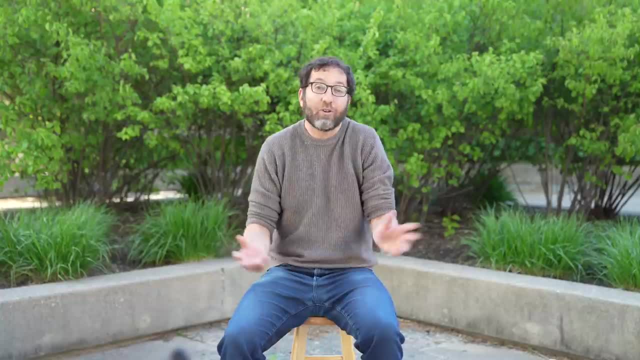 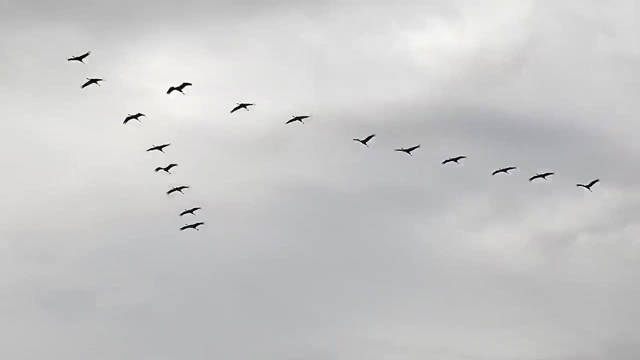 together. That was my way in. I still don't know where my office is. If I'm inside, I can find it. Don't worry, I know the number. That's how I find it. Geometry is everywhere. Any kind of game. 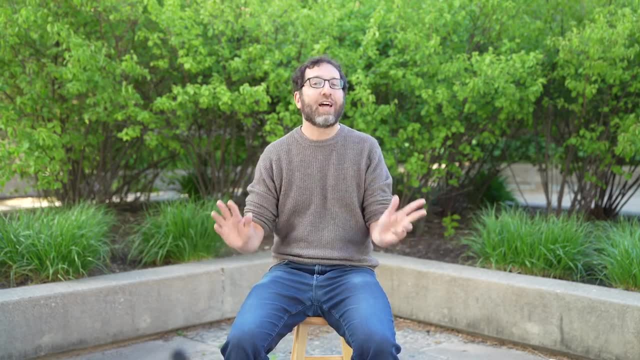 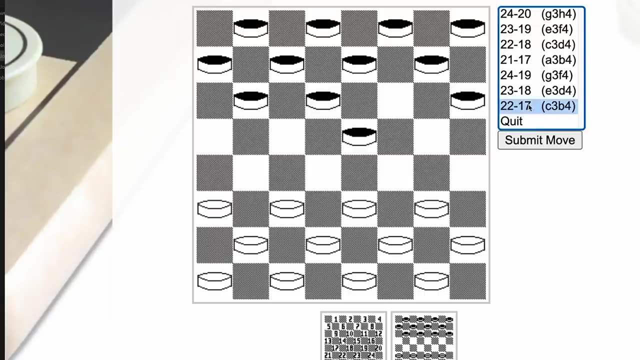 Whether it's checkers or tic-tac-toe or connect four or chess or go or whatever, the game itself has a geometry And when you train a machine to play that game, you're training the machine to explore that geometry, And that geometry is the geometry of a tree A. 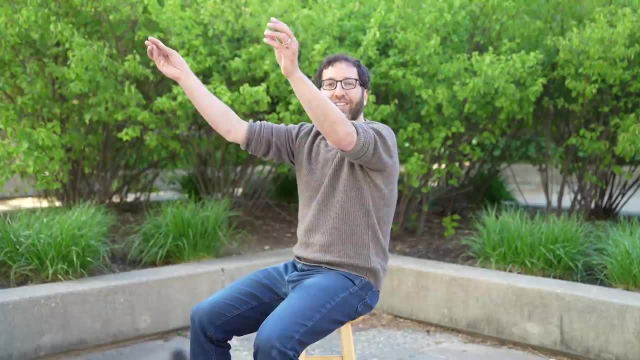 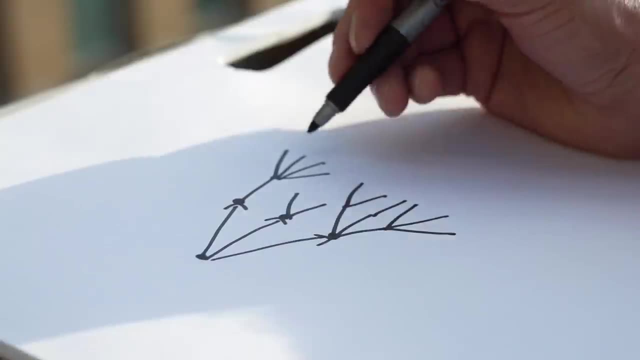 tree, depending on which one you look at, it has a trunk, and that trunk branches into smaller branches and the small branches branch into smaller branches, and et cetera, et cetera, et cetera. But you can never go back right. That's the way a game works. That's the way 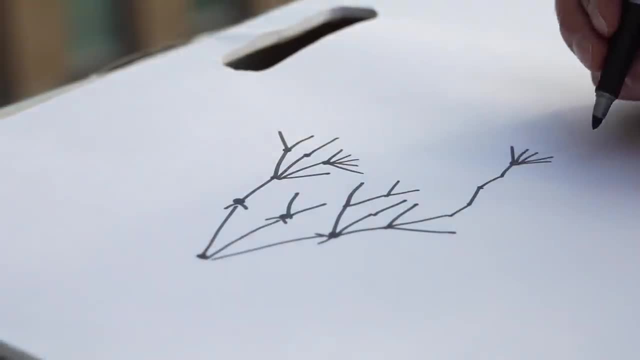 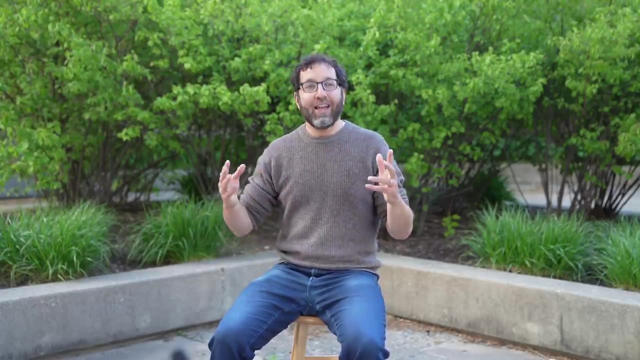 any kind of linearly sequenced set of decisions works. Subtitles by the Amaraorg community. It's the tree-ness of the geometry that makes those games solvable. That's what makes it possible for there to be a literally perfect strategy, which is what we now have in computer. 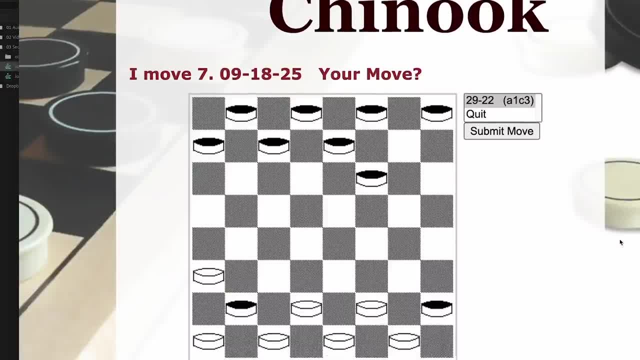 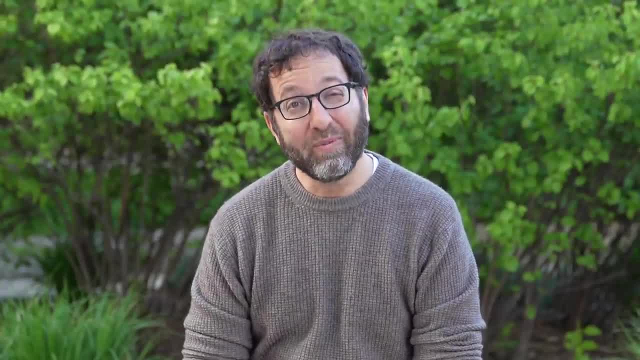 checkers So you can play against the computer. It's just sitting there at the University of Alberta running all day and night and you can log in and play against it At some point. usually it takes about three or four moves for me because I don't really know checkers. 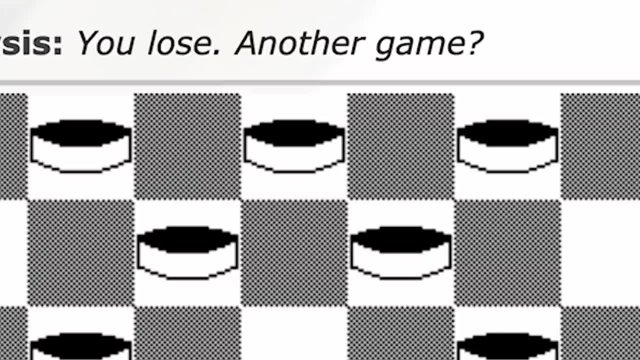 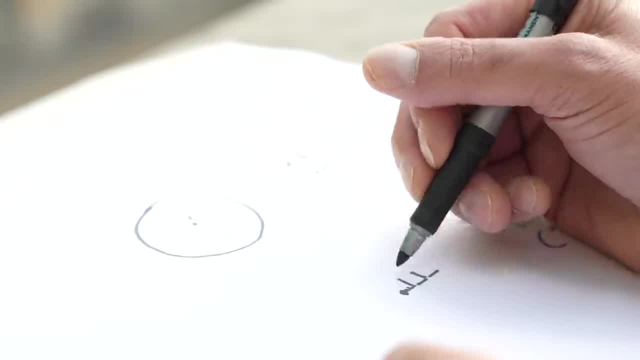 very well, It'll just be like I have one. If what you know about geometry is like the ninth grade, it doesn't seem like it could be very dangerous, but there's like a long history of seeing it that way. Geometry kind of creates a new locus of authority, that's. 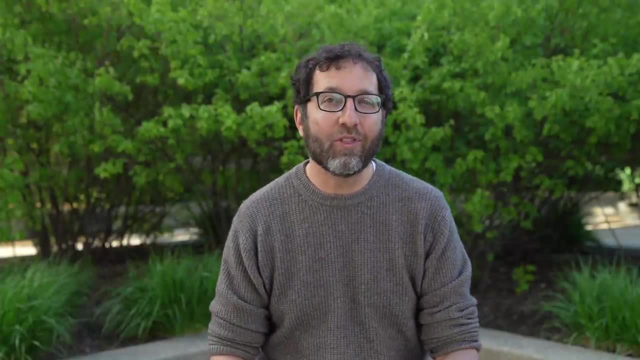 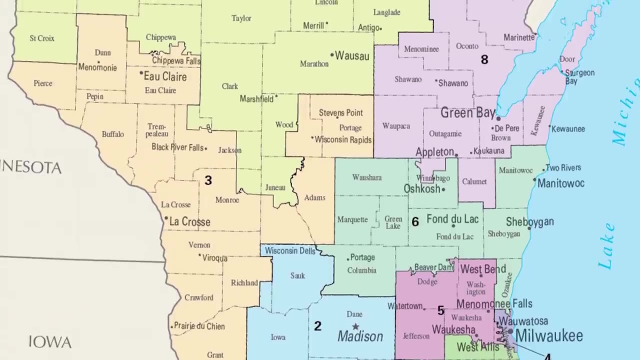 not under political control And lots of people see that as a threat. I mean there's this question about drawing legislative districts, which is such a hot political topic here in Wisconsin. Somebody's got to kind of sit down and cut Wisconsin into 99 parts, It seems. 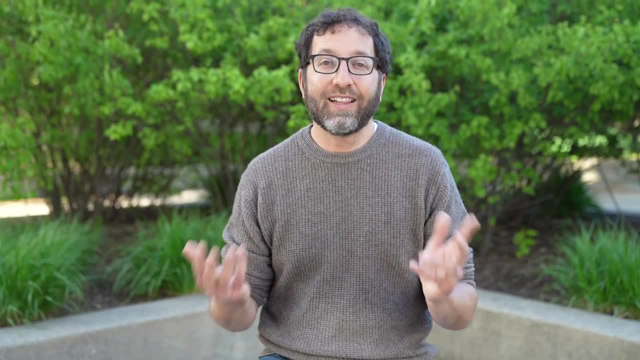 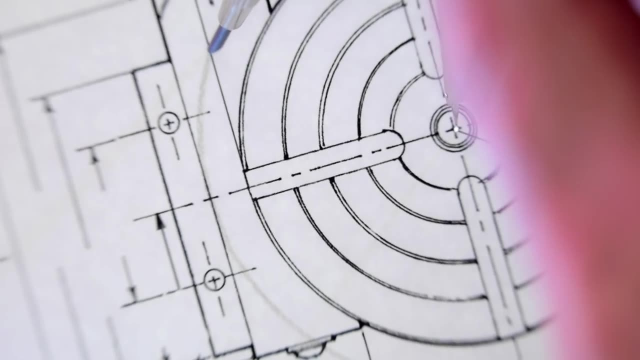 like a technical exercise, but it actually has a huge effect on who's sitting in a legislature, who's making the laws and, in particular, who draws the next set of lines. So there's kind of a feedback: If you're like me, right, if you're training math at first, you're like okay. so there's. 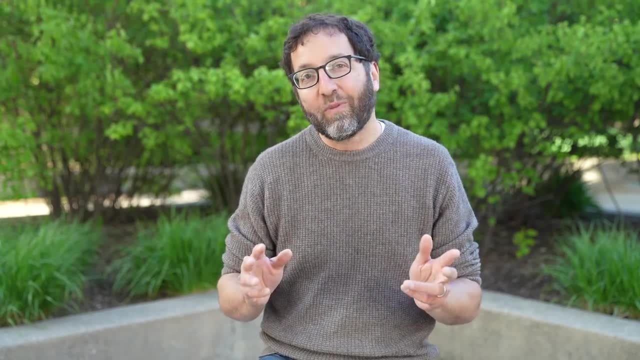 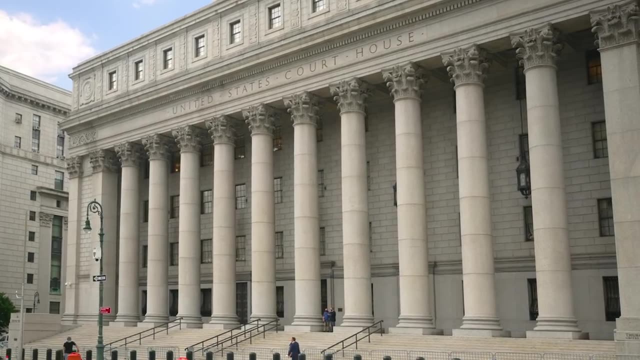 a math question here, Like what's the right way? It's not a math question, but it's not not a math question. The math is wound up with these political questions, with legal questions, which obviously are really important, but also with fundamentally philosophical questions.